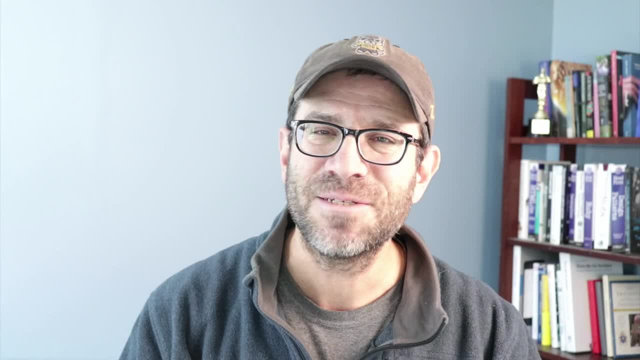 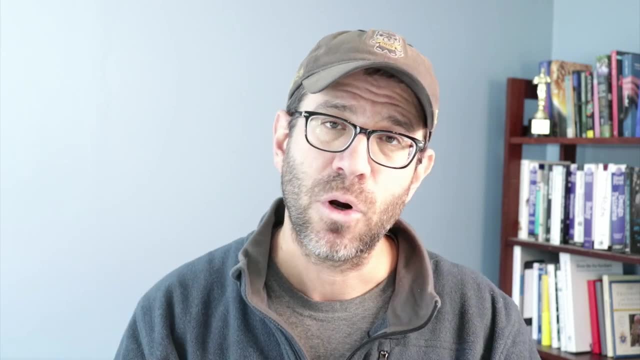 function name wherever I want to say, read in a file-up formatted distance matrix and I will then get that functionality. And so I want to spend a little bit more time in today's episode helping you to develop some more concepts and understanding of how functions work and how you. 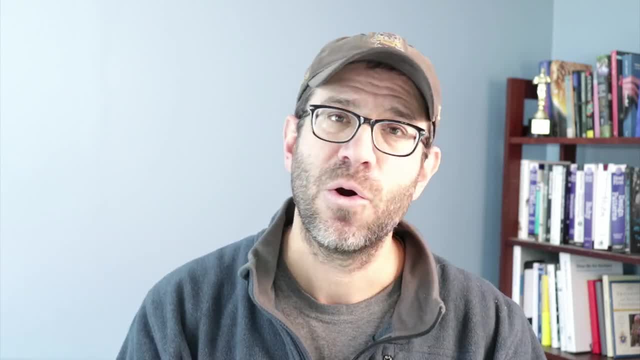 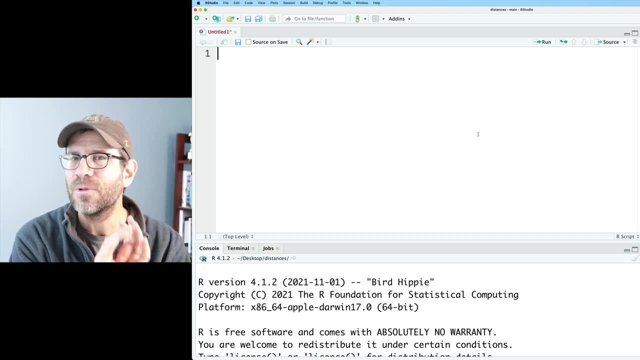 can write your own functions to help keep your code as dry as possible. Before we convert our code for reading in a distance matrix to a function, I want to start with a little bit of a little bit more simple example of functions to help relay some of the concepts that we need to 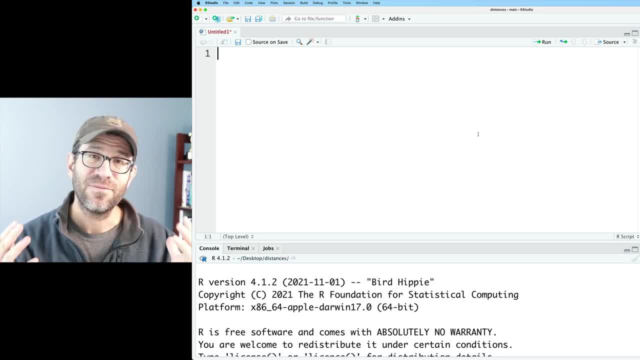 know, for creating our own functions. So the first thing that functions generally need is a name. So I'm going to create a function that converts degrees Celsius into Fahrenheit. I'm in the United States. We're like the only place in the world that uses Fahrenheit. I still don't have a 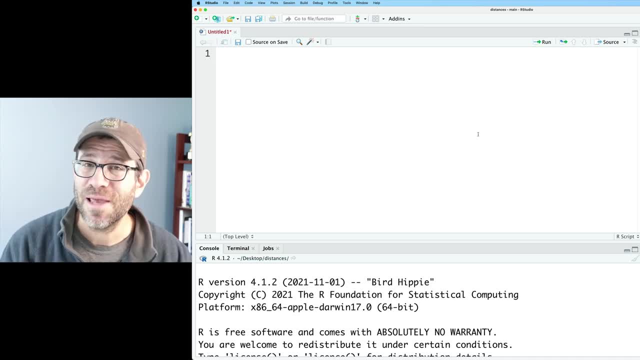 really good handle of what Celsius means, So such a function might actually be helpful to me. So I'll do C to F, And so C to F is the name of the function, And so C to F is the name of the function. 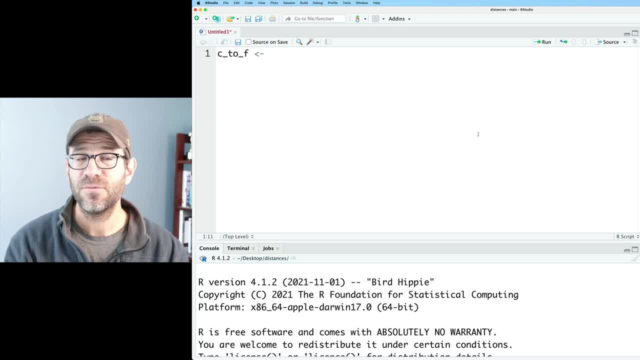 I like to have my function names be descriptive. So this is called snake case, where everything is lowercase And if you want a space you insert an underscore. You don't want to have hyphens, because a hyphen also means minus, And so if I had C hyphen two, hyphen F, it would think I would be. 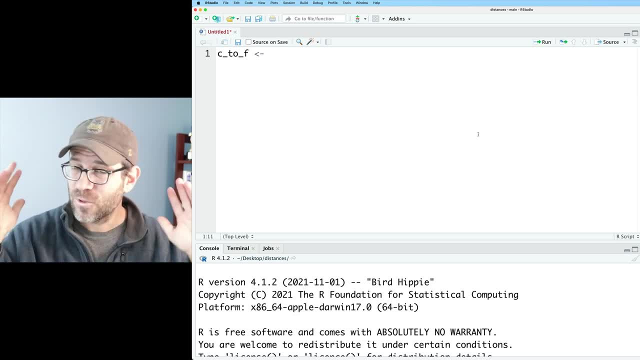 subtracting two from C and F from two right, Which is not what I want. I want it to be C to F, And so that is the name of my function. I then use that assignment arrow because I'm going to assign output of a function to that variable. And what is the name of that function? Well, it's function. 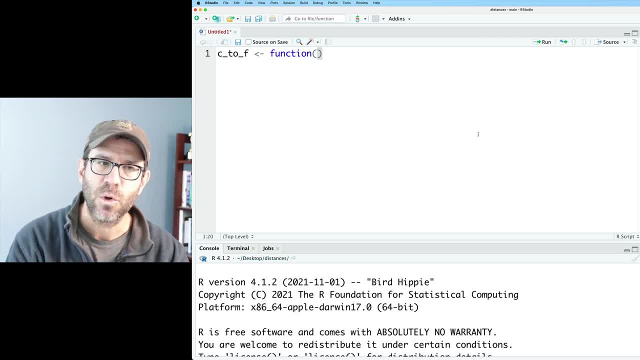 right, And so we are going to define a function using the function keyword, And so that function keyword is really important. And inside of those curved braces, those parentheses, we then put an argument list, And so what we might put in here then would be Celsius, And that would be my. 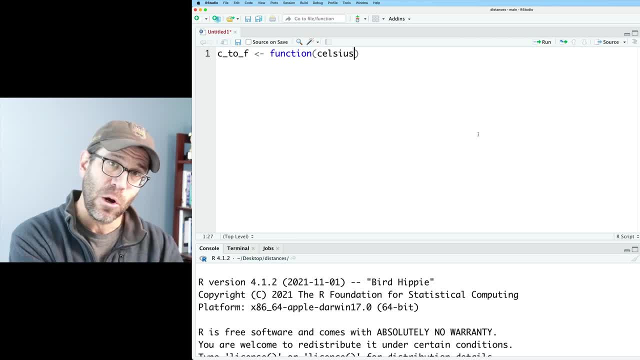 temperature, That would be the input in Celsius, And we're going to output Fahrenheit. So then, the next part of a function is the output of a function, And so we're going to put in here: the function is the body of the function. We will then give the special sauce, as I like to call it. 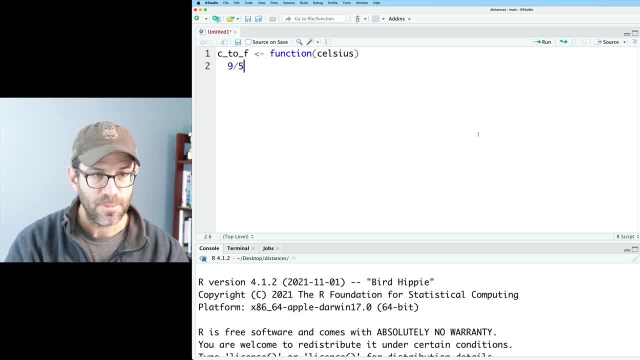 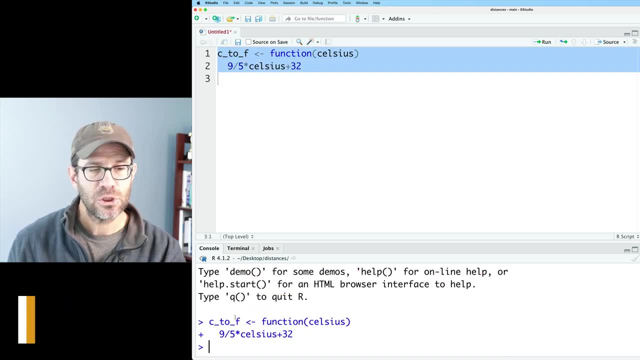 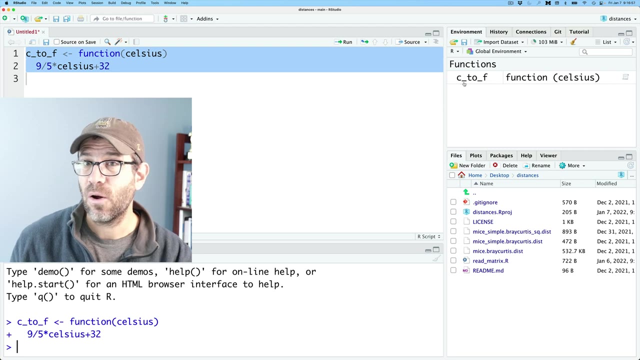 of what's going on, And so the conversion would be nine divided by five times Celsius plus 32.. And so if I want to load this, I then load it into my R session. If I look at the environment in the upper right corner of my R studio session, I see that I now have a function loaded C to F. 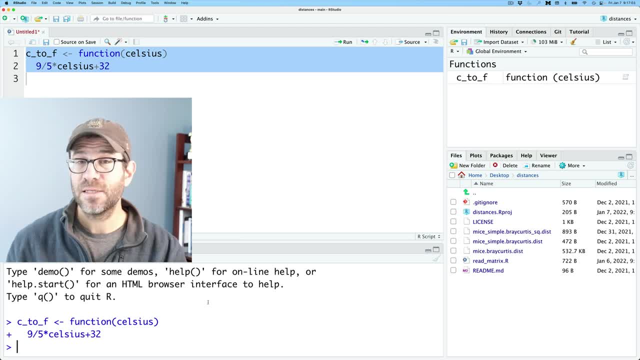 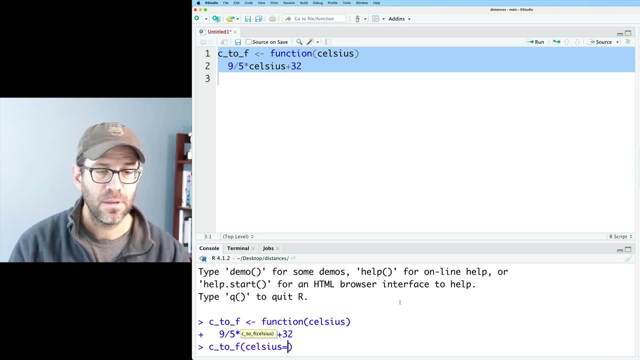 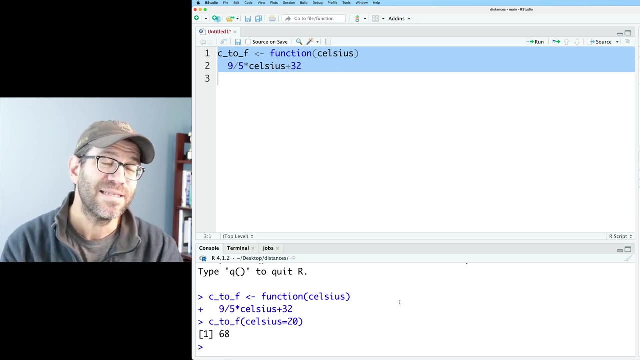 It's a function that takes in Celsius, right, And so then to call C, I can do C to F and I can give it a temperature right, So I could say Celsius equals 20. And so that would tell me it's 68 degrees Fahrenheit outside. Now there's a few nice things to know. 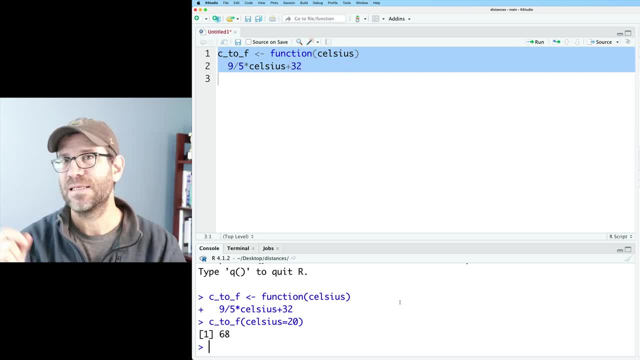 about running functions. I don't actually need to say: Celsius equals 20,, right? I could do C to F, 20, and it'll output 68. So R is smart enough to know that. if there's only one argument, Celsius. 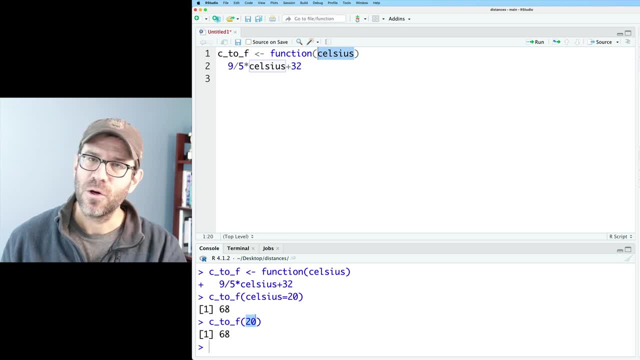 then that if I give it a value or an argument that that goes with the Celsius, Well, what happens if we have a couple arguments? So this is a little bit silly, but say I want to add freezing right, And that would be 32,. 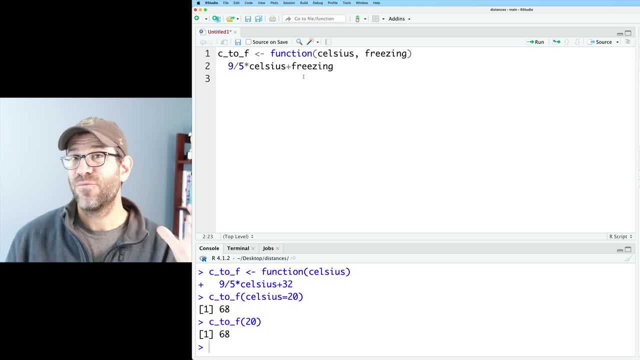 right, So I could then do freezing as another variable in my function. So I could then do C to F, 20,, 32, up. And I just fell into a trap that I commonly do, where I change the function but I forgot to reload it. And so that's an important point, that if we change the body, 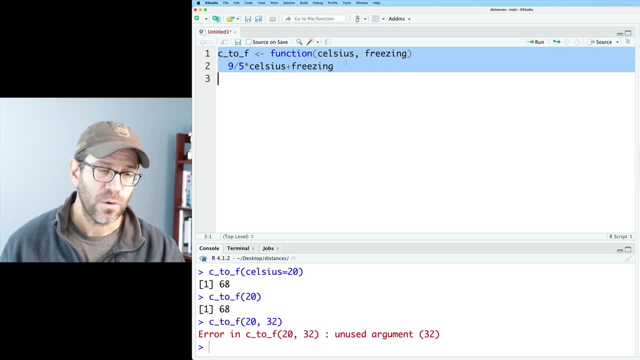 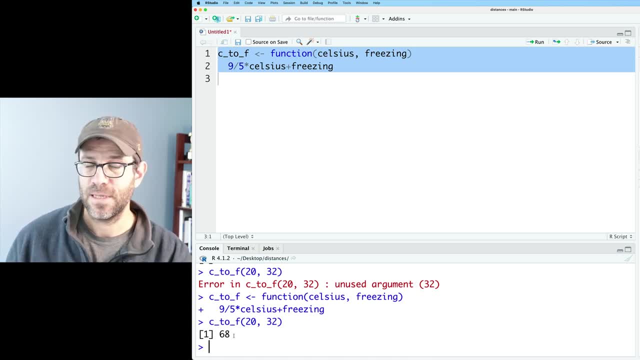 the code I get C to F, 20,, 32,, 68.. And you'll notice that again, I didn't put in the argument names And that's because R is being smart and that if I give it two arguments it knows the. 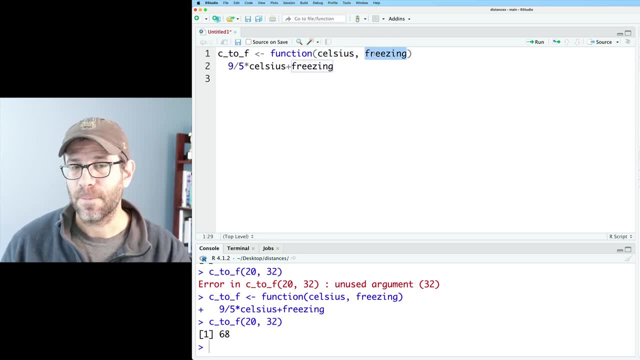 first argument goes for Celsius, and the second goes for freezing. What it's not smart enough to do, though, is to change the arguments of our function so that we can then go ahead and use C to F, 32,, 20,. it's not going to give me 68. Because, again, it's assuming that first value 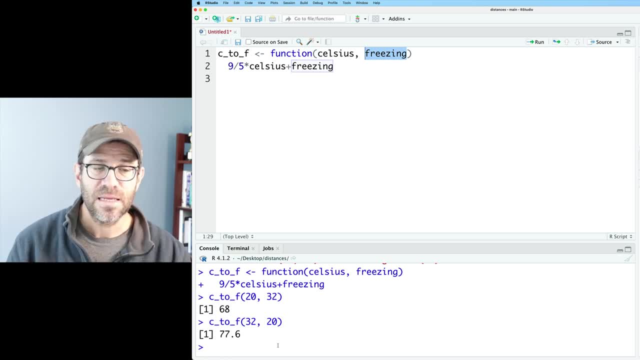 is Celsius and the second is freezing. That's not the case. If I wanted to do something like this, where I do 32, 20, I could do: freezing equals 32,, Celsius equals 20.. And that way it is telling R. 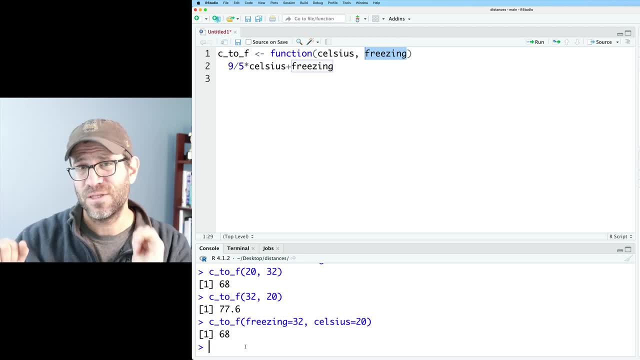 okay, I don't know the order of the arguments, but I want the freezing to be 32, and Celsius to be 20.. And you can get a little bit of a difference there. So if I do C to F, 32,, 20,, it's not going to give me. 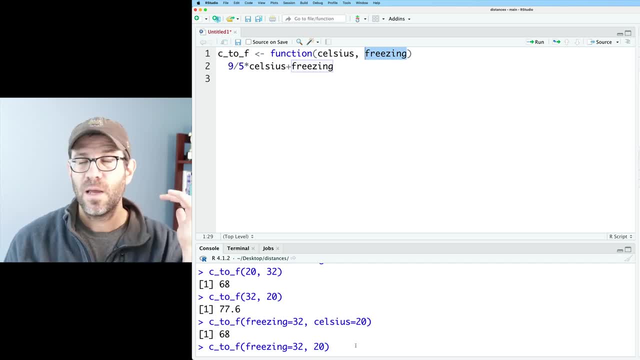 32,, 30,, and I want the freezing to be 32, and Celsius to be 20.. And so I'm going to do this a little bit silly with some of this: Say, I wanted freezing to be 32, and Celsius to be 20.. If I know. 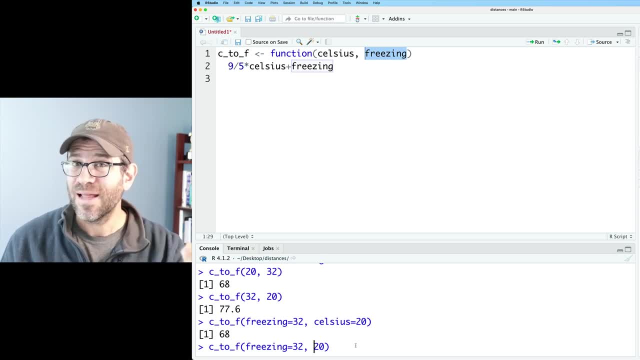 there's only two arguments. I can say: freezing equals 32, and then not label Celsius for 20, and I'll get back 68.. So again, R is smart enough to figure this all out, thankfully Now, of course. 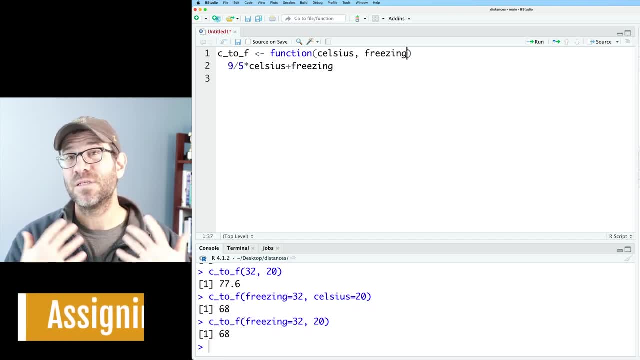 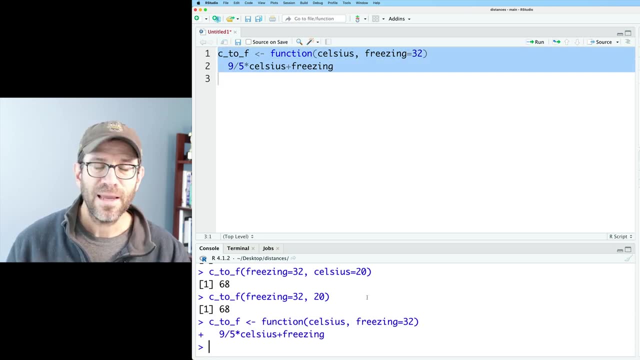 freezing is always going to be 32 in my case, And so I might like to use a default value for freezing, So I could say: freezing equals 32.. And so again, if I reload this, I can again do C to F. 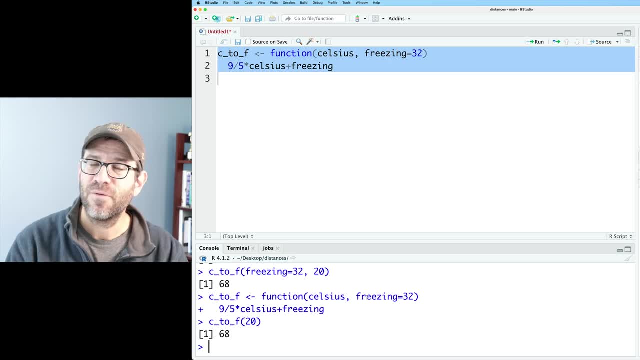 on 20, and it should be 68. And sure enough it is because it's using the default value of freezing to do the calculation. Of course I could come back and use freezing 32, and Celsius 20, like this, and I get the same thing. So say I want to do something a little weird and do C to F. 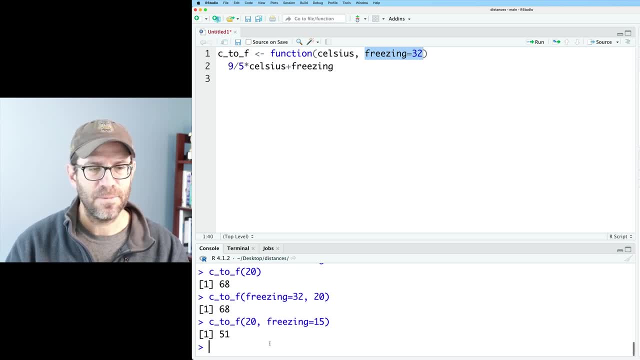 20, and then freezing equals 15,. I would then get back 51. Again, this is also a very simple one line function. Let me show you what we would do if the function were perhaps a little bit more complicated. Well, if we had more than one line in the body of our function, 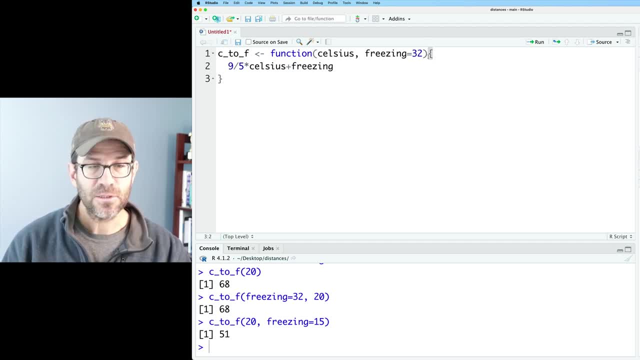 we would need to use a set of curly braces, And these are the keys to the right of the P on your keyboard. when you hit shift, Those give you the curly braces, And that curly brace defines the body of your function right. And so again, I can run all this, And if I do C to F on 20,. 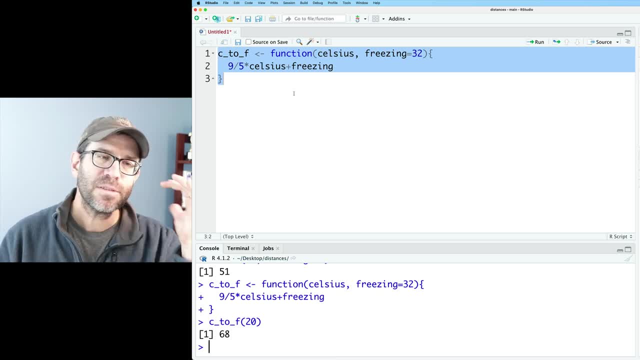 we should get back 68, our good old friend right, And so what this allows us to do is to have multiple lines in the body of our function. I'd be pretty hard-pressed to come up with an example where I don't use the curly braces to define the body of a function. 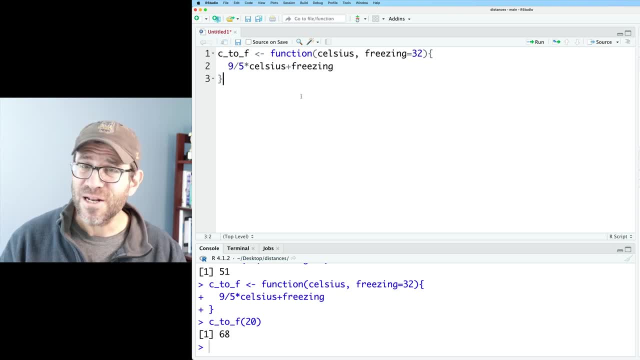 Generally, my functions are going to be more complicated than a single line eventually, If not from the beginning, then yeah, like I said, eventually they will get to be multiple lines, And so it's nice to, from the outset, define the body of the function with those curly braces. 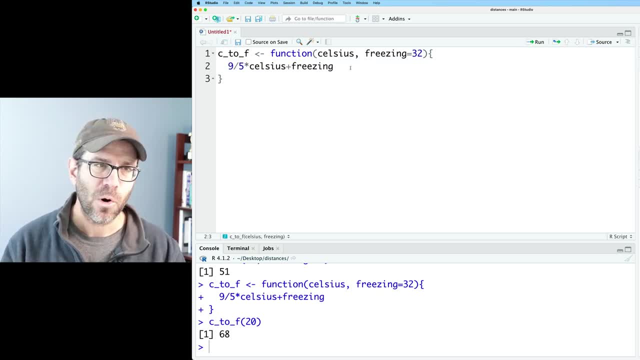 So to help flesh out what this might look like if we get things a little bit more complicated, let me break this equation. And so here we'll do multiplication as the 9 fifths times Celsius, And then we'll do multiplication plus freezing. Again, I'll highlight and run all that And we'll again. 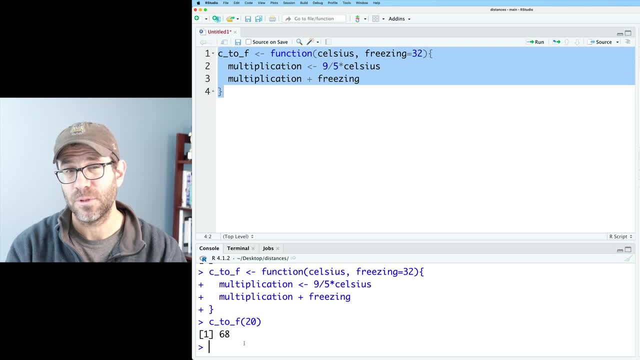 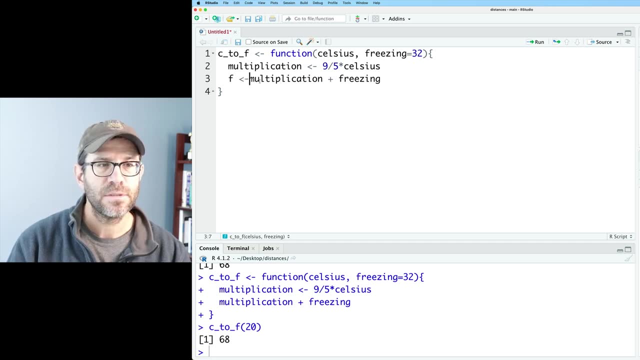 do the C to F 20, and we'll get back that 68, right? So again we can have multiple lines in here. So generally you might start assigning values to variables as the code gets more complicated, And so I could assign this multiplication plus freezing to the variable F. 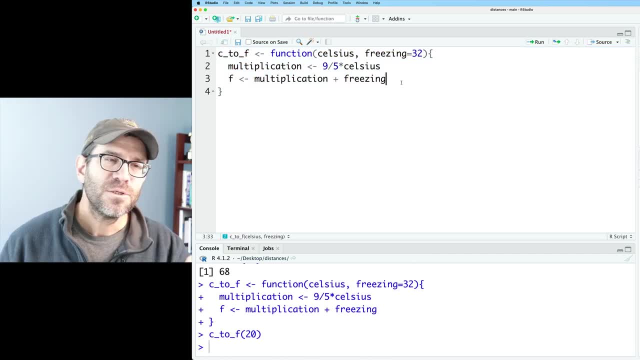 and so now, if I do C to F, I don't get any output. To this point we haven't been assigning the output within our function to a variable name, And so the function returns the last outputted value. What we did here on line three is we took multiplication plus freezing and assigned it to 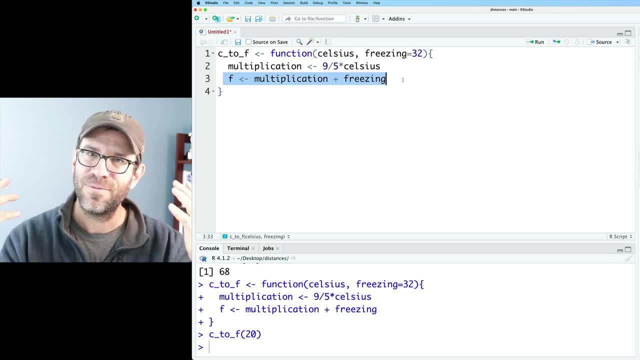 the value F, And so that is the last executed result inside of our function, And so that doesn't really have a numerical value. that's getting outputted to the main session in R. What we could do is we could say F, right, And so now the last outputted thing from the function will be the. 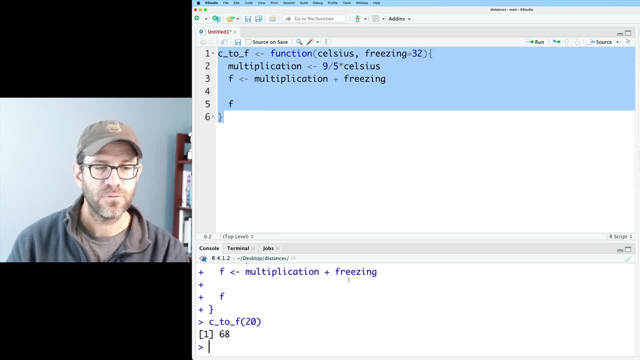 variable F. So now, if I do C to F 20, I get back that 68.. Alternatively, what we could do instead of listing the variable itself, which is a little bit more elegant, is to say return F, And so this: 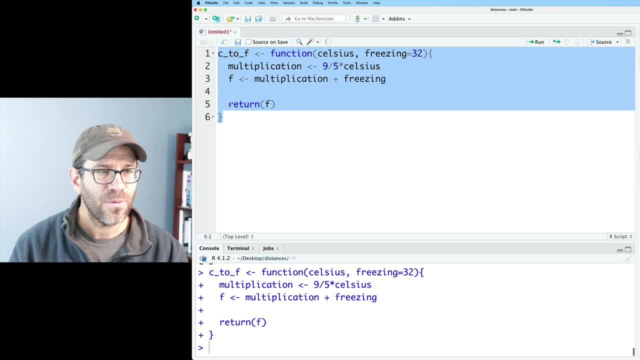 is telling R return F. So now when I run this again, if I do C to F, 20, I get back that 68.. One thing that's important to know about the return function is that it's not going to return the. 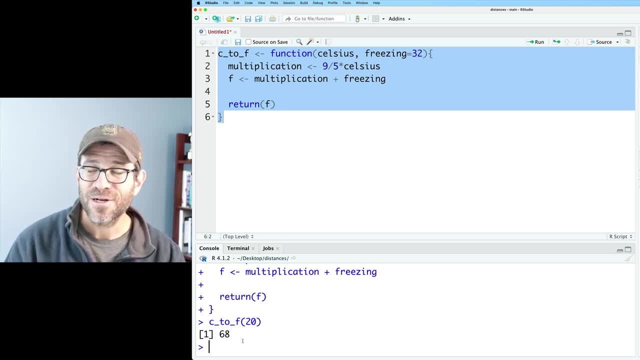 function, however, is that if you put that return function anywhere but the end, then everything after the return function will not get run. So of course we'd want return F to be the last executed code in our function, because we know that when it runs return, it's going to kick out. 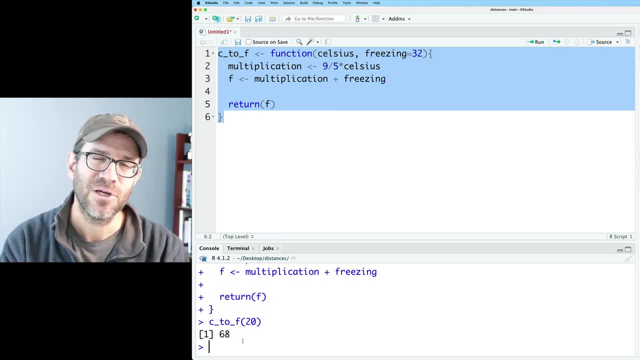 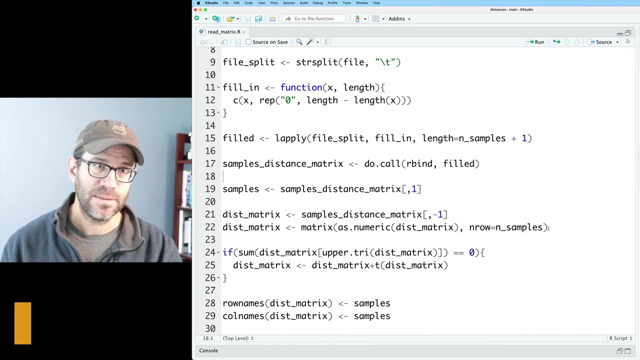 of the function. Okay, so that's enough to cover here in talking about functions. Let's head over to the code that we've been working on to build out that function for reading in a file formatted distance matrix. Let's look at our code that we've been developing for reading in a file up formatted distance. 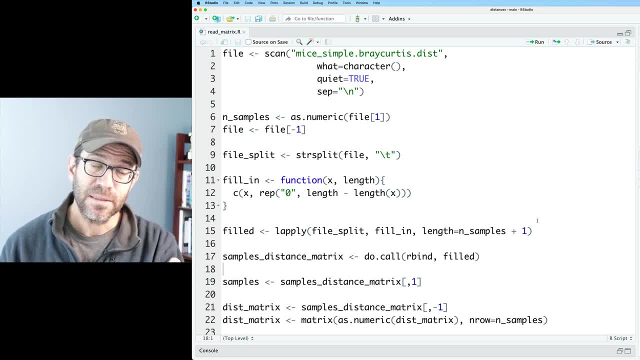 matrix here in read matrix R. If you want to get this code down below there is a link that you can go to to get this file as well as the data that I am working with. So, again, this is kind of a stream of consciousness code And, as I said before, I could change the distance matrix that I'm 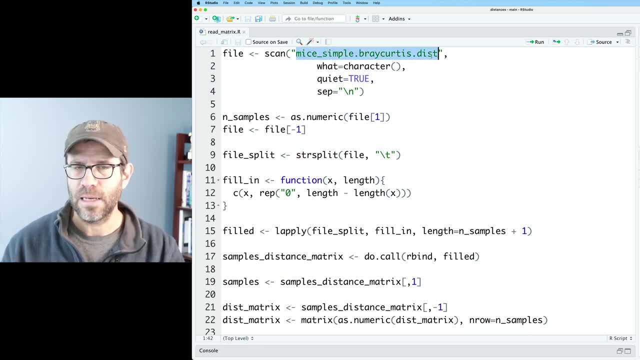 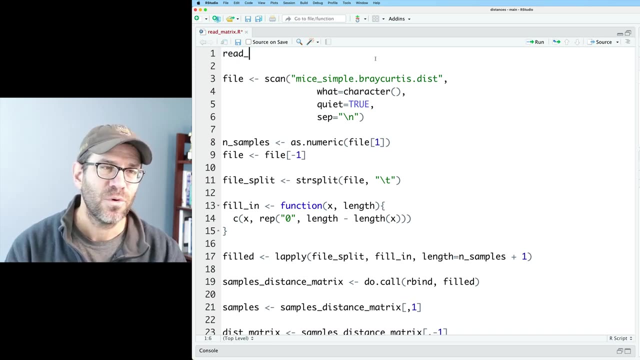 reading in by changing what file I am reading in, And so I want to make this dry, So I'm going to do that. I'm not repeating this every time I have a different distance matrix that I want to read in, So I want to turn this into a function, So we need a function name, And so what I will call this is: 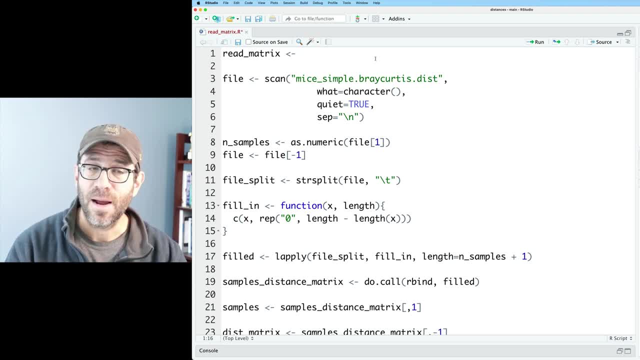 read matrix And we again use that assignment operator and then the function keyword And we're going to give it one argument and that is going to be the file name. And again I like to use descriptive file names as well as function names. My file names are generally nouns and my 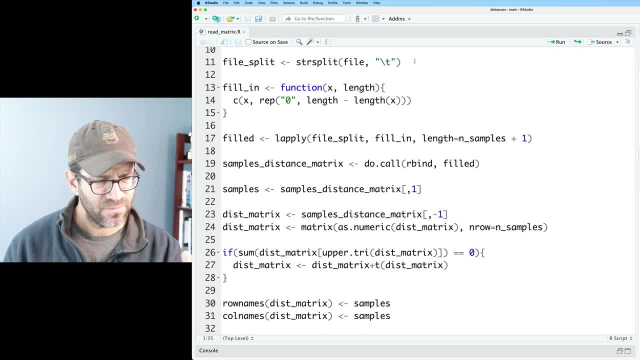 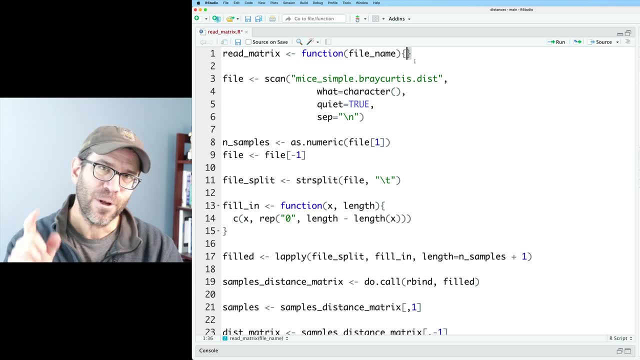 function names are generally verbs, like what is happening, right? So I have 31 lines of code, So I need to insert those curly braces to define the body of my function. In RStudio, if I put in the open curly brace, it automatically gives me that closing curly brace. So I'll go ahead for now and 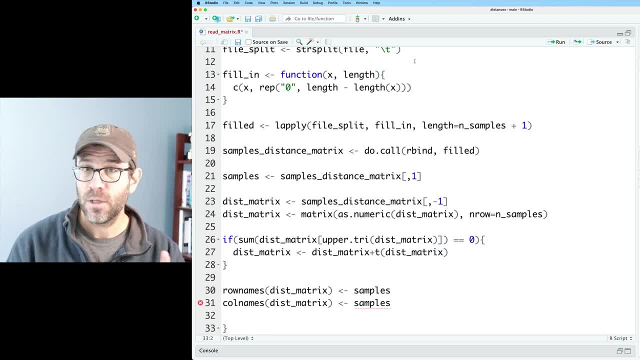 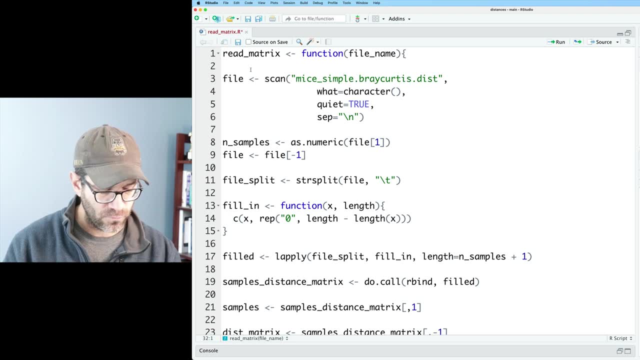 delete that closing curly brace, come to the end and put in the closing curly brace. One of the things I also like to do in functions is in the body of my function. I want everything indented over a notch So I can highlight all the code. 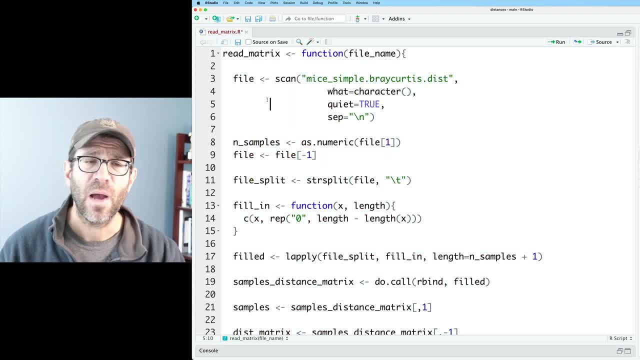 delete the tab and it'll go over two spaces or whatever. you have a tab defined as in your settings for RStudio, So great, we have a function. But, as I said, I want to replace this file name with the variable file name Because, as a user, when I call read matrix, I'm going to give it my 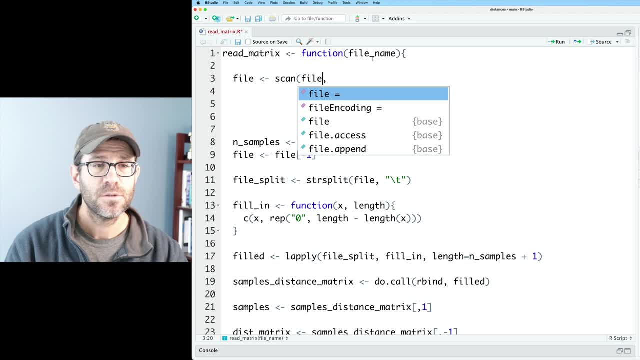 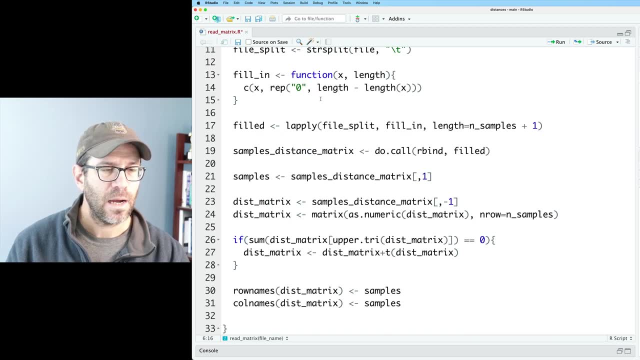 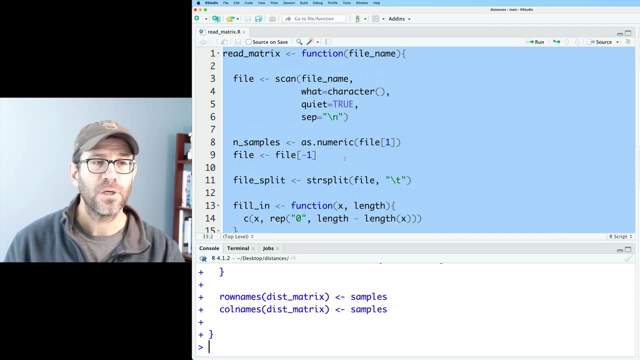 simple break-curtis, dist or whatever distance matrix I want to use. So I will then put in file name And maybe I'll go ahead and clean up my tabs here And so that all looks good. So I'm going to go ahead and save this And I will run this so that I now have read matrix in my environment And 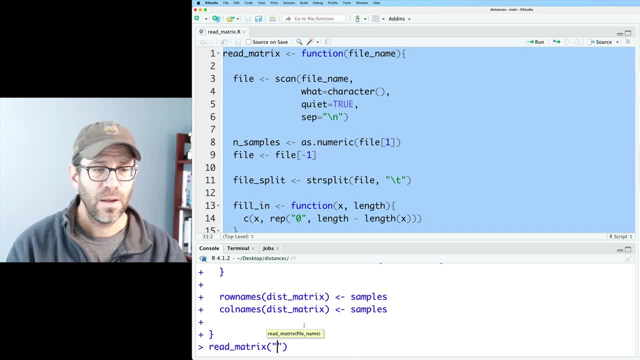 I can do read matrix, And then I can do mice, simple break-curtis dot dist, And I'll run that And I don't get any output. Why don't I get any output? Well, perhaps you've noticed the last two. 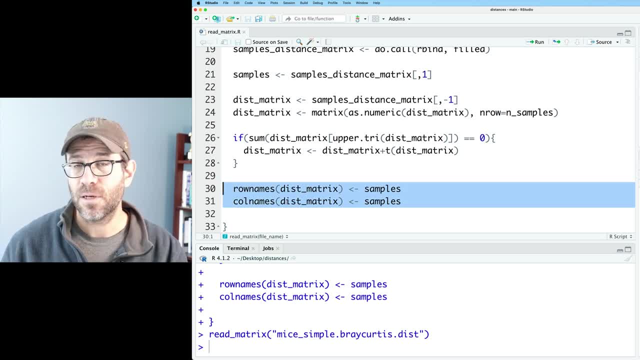 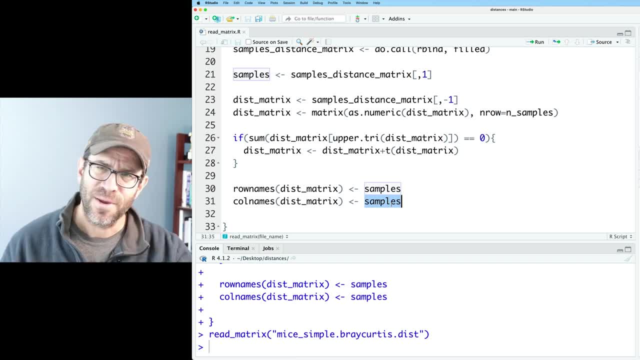 And it assigns it to the row names and column names of the distance matrix. This is what we covered in the last episode. Well, that's not generating any output to the screen, So nothing is getting returned from the function. So again, I could do dist matrix, But I'd rather do return. 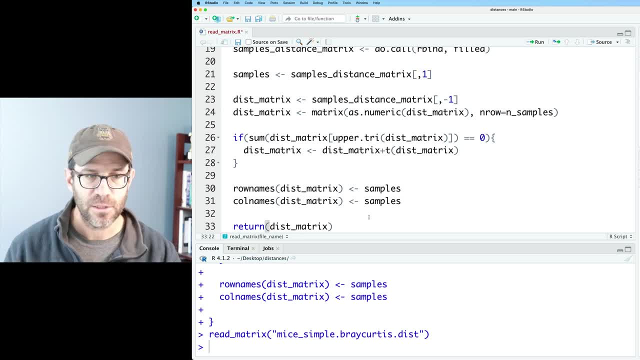 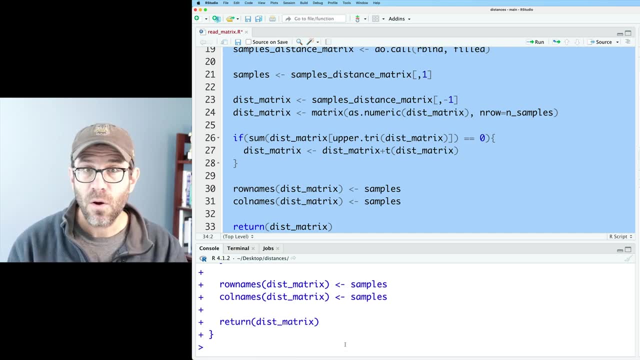 dist matrix to make it more explicit what's happening here in the function. So because I've modified the code, I need to go ahead and highlight everything, reload it into R, And so now I can do read matrix And then I can do the function, And then I can do the function And 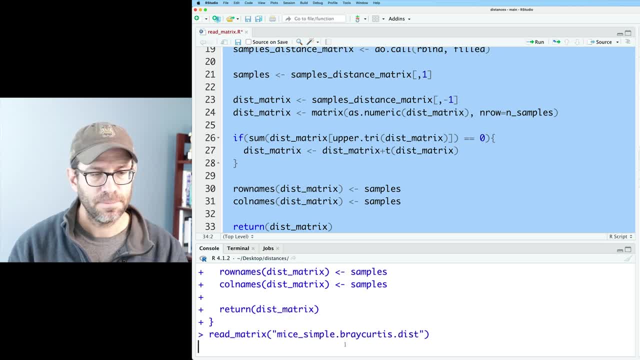 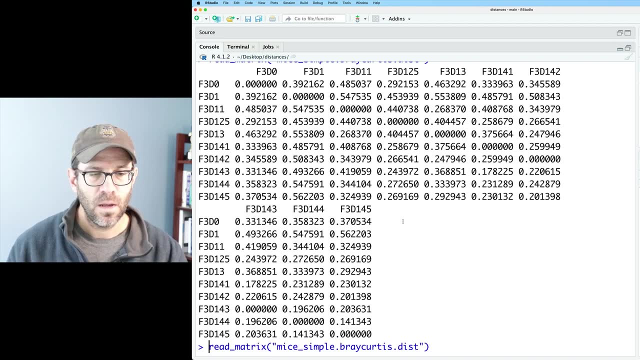 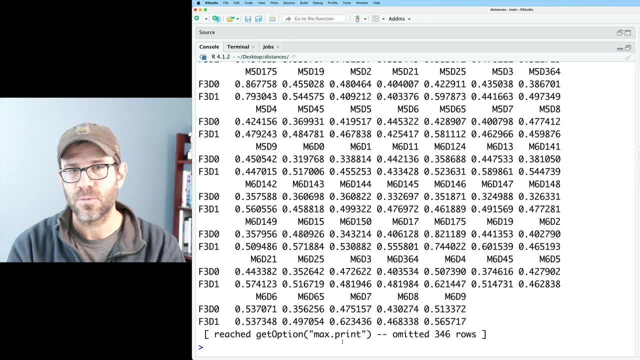 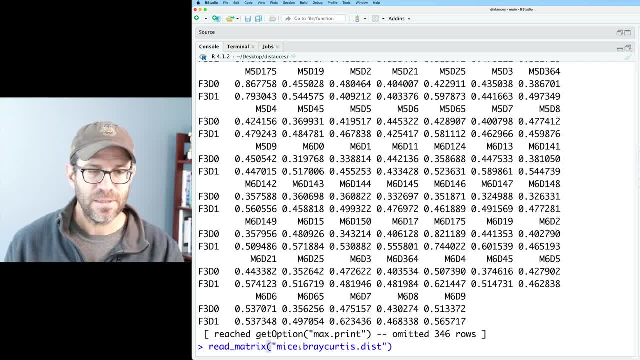 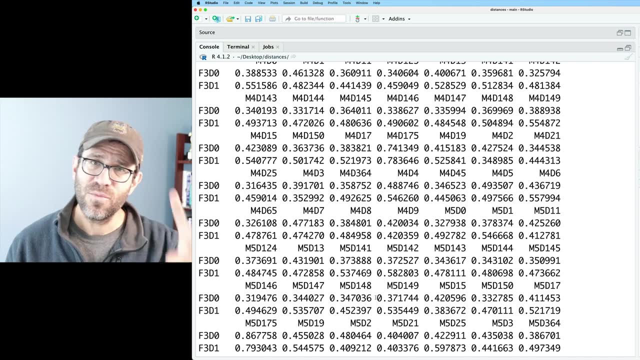 the rows because this distance matrix is much larger. But you can see that I can read in these different distance matrices with running the same function but giving it different file names. So here I've created distance matrices from three different files without having to rerun those 30-some lines of code. 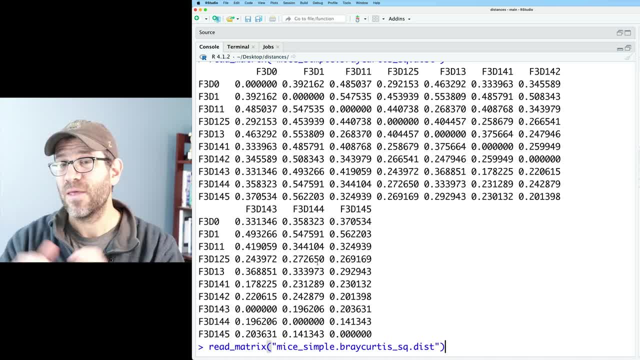 All I had to do was run readmatrix, parentheses, and the name of the distance matrix file that I want to read in. Of course, I could then also assign this to a variable, So I could then say: distmatrix equals readmatrix and the file name. 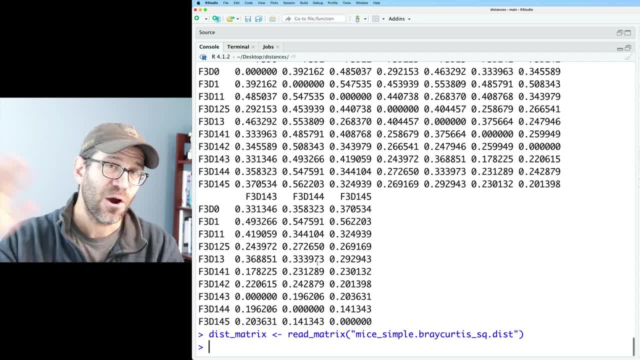 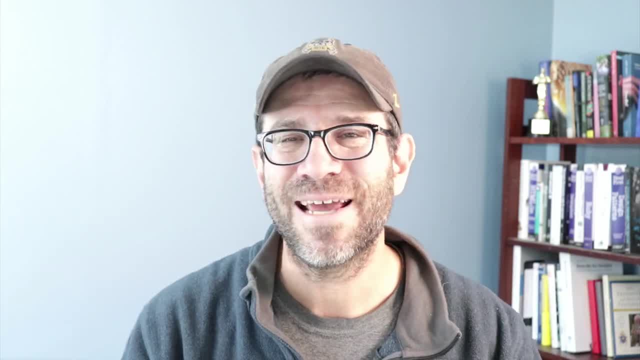 And so now distmatrix contains that distance matrix And I can go forth and do all sorts of cool things that will happen in the next episodes of Code Club. So you know what happens in those next episodes of Code Club. I'd love it if you made sure that you've 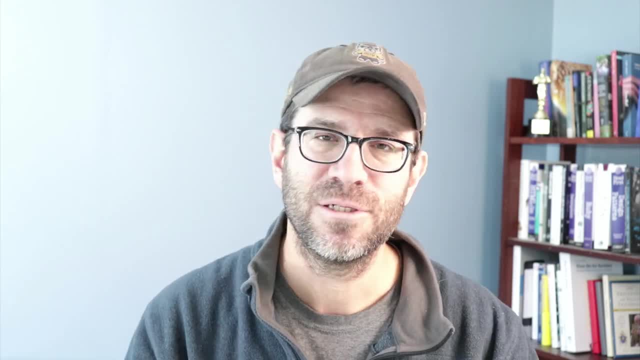 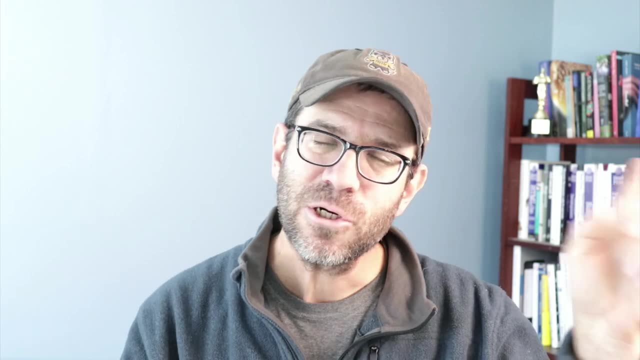 subscribed to this channel. you click the bell so you get the notifications of when things happen And really we are on a journey here And if you're just joining us, welcome. Please be sure to check out the playlist that I have up here. 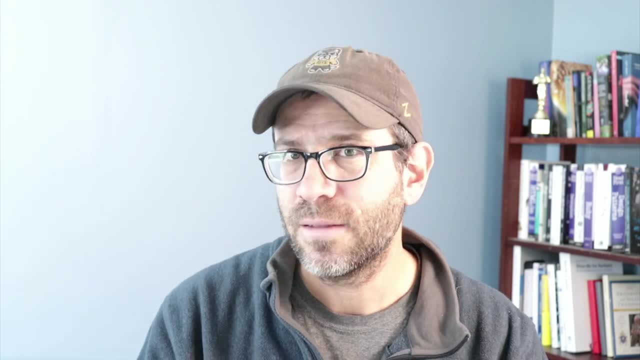 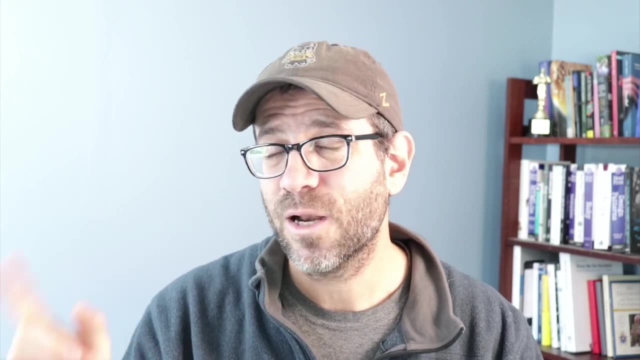 and encourage you to go back and see how we've gotten to this point in this development of this current series Moving forward. we're going to talk about a few more things having to do with base R, But eventually we're going to move on.